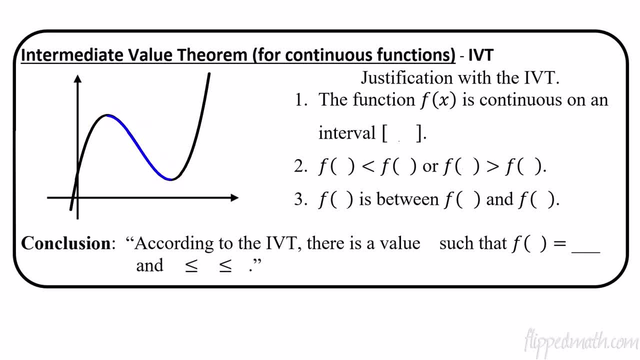 just this piece right here, from this maximum to this minimum. So what you're going to draw is just something that looks like this, but maybe you could draw it a little bit larger, just to kind of take up more room, maybe something like that. So we're focused. 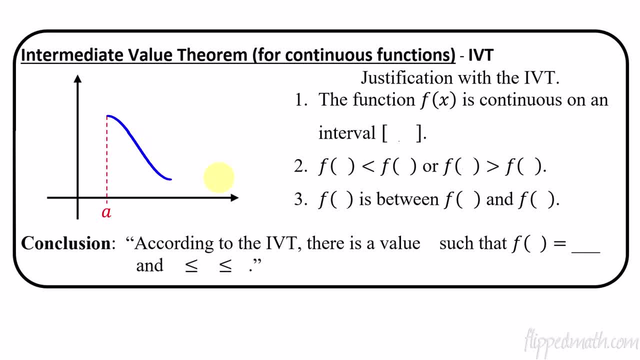 in on one part of this polynomial graph and I'm going to label the beginning point as an x value of a and the end of it an x value of b. So we're on the interval a to b. So what we're looking at is that, the function to use. 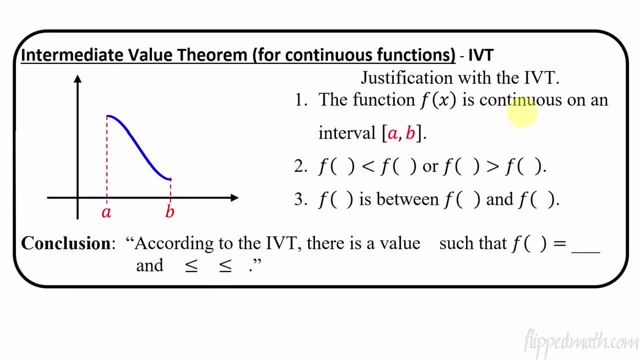 the intermediate value theorem, the function must be continuous on an interval from a to b. So that's one of the conditions that we must meet in order to use the abbreviation IVT, the intermediate value theorem. So next up, if this point right here. 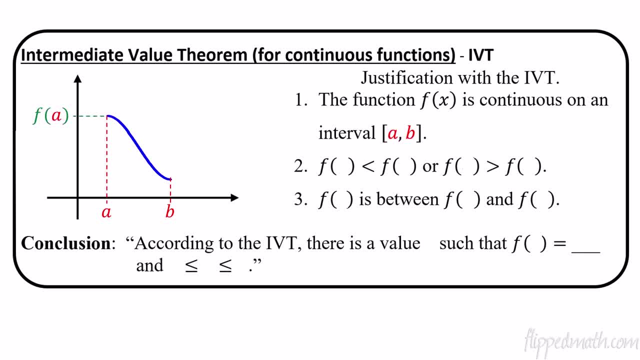 is x equals a, then what is the y value? right there, It is f of a, And if this is x equals b, then of course the y value would be f of b. So we have x values, y values. Now over here what that leads us to. 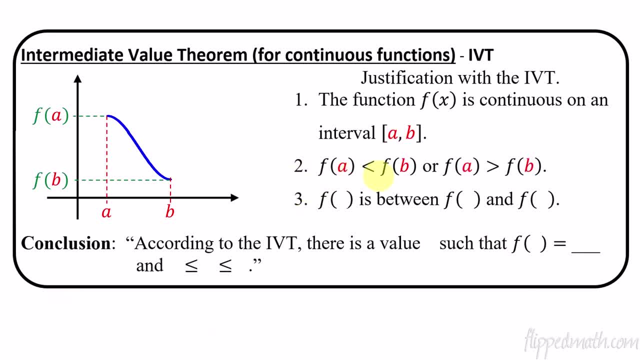 is that we're going to have: f of a is going to be smaller than f of b or it's larger than f of b. In other words, the two y values are just going to be one's larger, one's smaller. That's all we're. 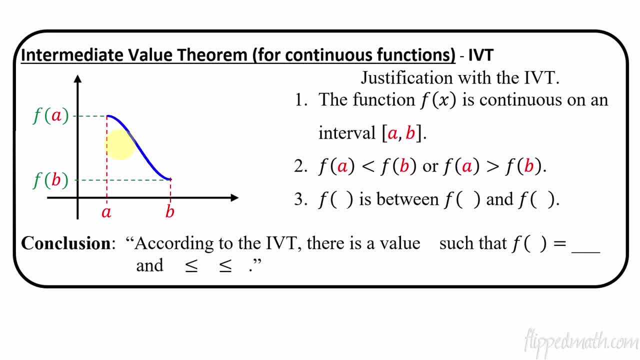 looking at. So for the intermediate value theorem to work, it's got to be continuous. and then the y values of the endpoints. one has to be smaller than the other. Next thing I'm going to do is I'm going to throw in a random letter c. 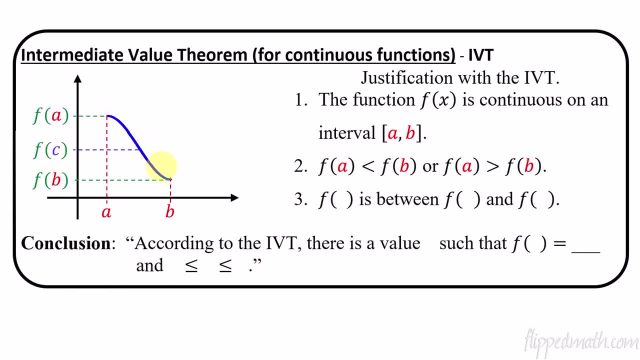 So f of c, some y value somewhere in between f of a and f of b, Some random point. Now, what I know about that is that that means that f of c is in between f of a and f of b. Once we have all this set up, we can then say that there's 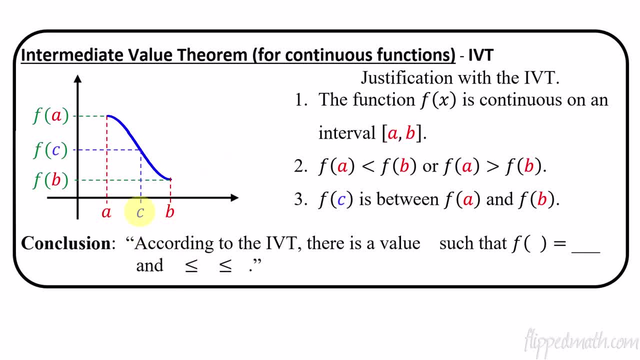 got to be some value c in between a and b. Okay, so watch this. According to the intermediate value theorem, there is a value c right there, such that f of c is going to be a value c To equal, and then this is where I'm going to put a little question mark. this will 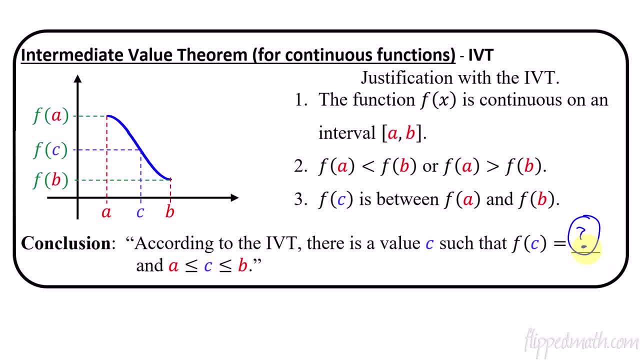 change for every problem. It's going to be whatever the problem's asking us for, whatever number it is. You'll see when I use this conclusion here. you'll see on some of these other problems. So there's a value c such that f of c has to equal some. 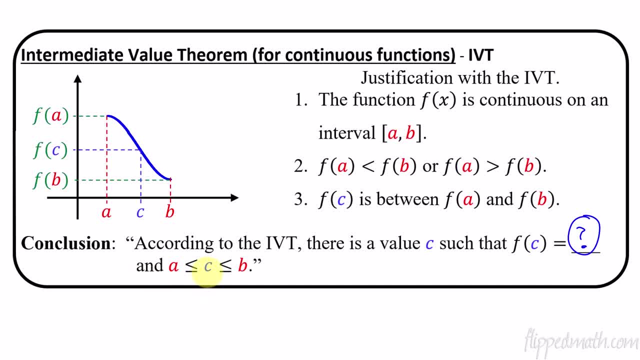 number, and that that letter c or the number c, I should say, is inside the interval a and b. Okay, so that might look a little confusing, but let me show you how a lot of it is just common sense. and then we're just. 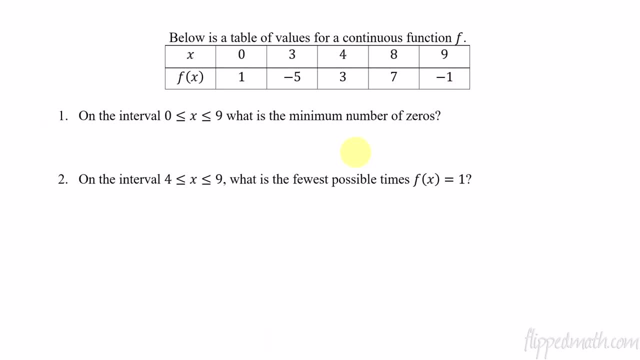 going to practice with the justification. So for this one, on the interval 0 to 9, what is the minimum number of 0s? And a 0 means when the y value is a 0. That's what we're talking about with 0s. 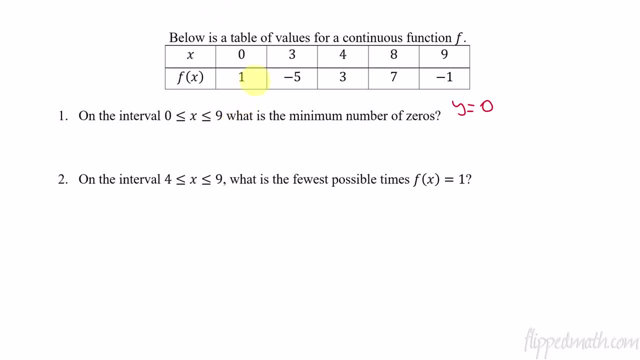 So, interval from 0 to 9, what's the minimum number of 0s? Well, let's see here We're going to go from 1 to negative 5.. So in this interval, at some point this thing has to cross 0. There's going to be a 0, right there? 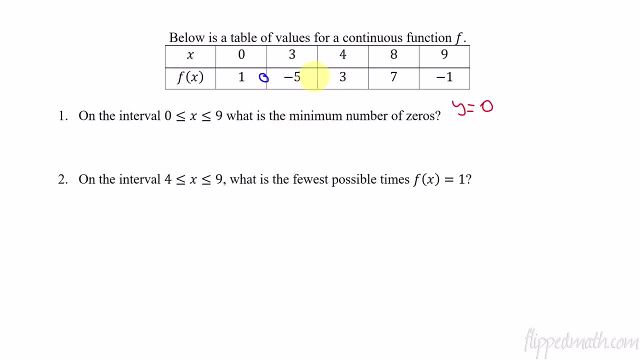 And then from negative 5 to 3,. again we're going from negative to positive. so there's got to be a 0 right there. From 3 to 7, there's no guarantee of a 0. There might be. It might dip way down below 0.. 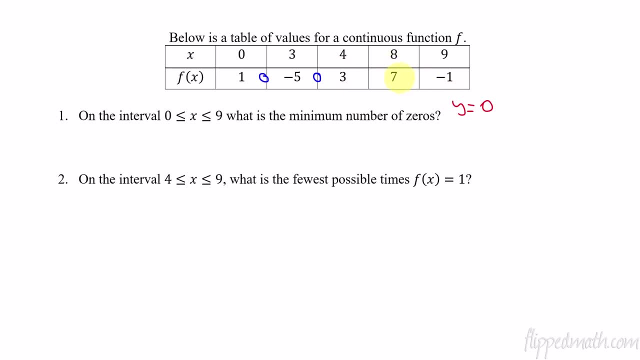 And then come back up to 7, but we don't know for sure. And then here, from 7 to negative 1, there has to be a 0. So we're guaranteed to have 3 0s. Okay, I don't have any explanation here and I'm 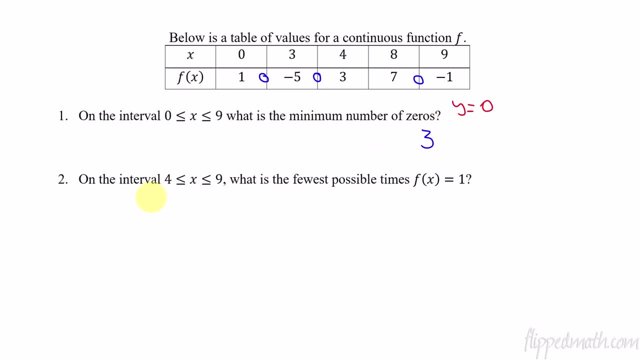 justifying it. I'm just kind of saying what the minimum number is. Alright, how about this one On the interval from 4 to 9, what is the fewest possible times? f of x has to equal 1?. So if we're going from, I'm going to erase this, so it's not there. 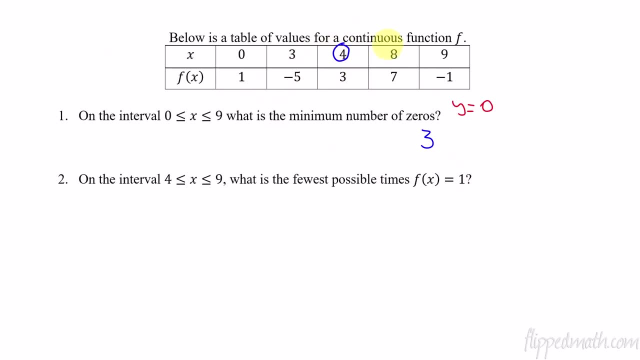 anymore. So from 4 right here until we get to 9.. So from there to there, how many times does it must equal 1? If we start at 3 and go up to 7, there's no guarantee that a y value is going to be 1.. But from here, from 7 to. 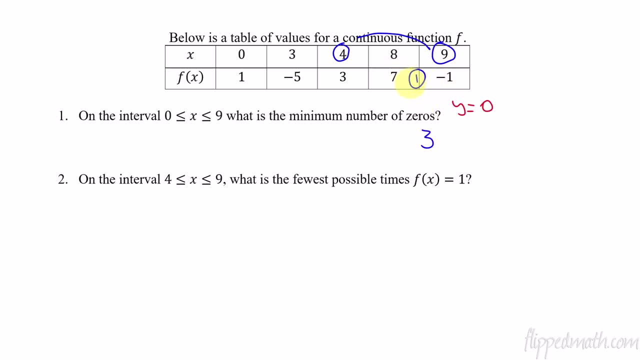 negative 1, we're going to cross that line of 1.. You're going to have a 1 somewhere in between there, So what is the fewest possible times It's going to have to at least show up one time right there, And I'm not justifying this again. 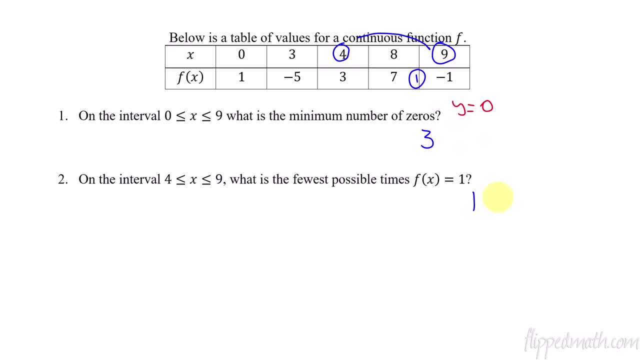 I'm just kind of stating the obvious. I'm just getting you to practice thinking about intermediate value theorem, that all the values that are in between 3, 7, negative 1, have to equal 1.. So from there to there, how many times does it must equal 1?? If we start at 3 and go up to 7, there's no guarantee that a y value is going to be 1.. So from there to there, how many times does it must equal 1?? If we start at 3 and go up to 7, there's no guarantee that a y value is going to be 1.. So from there to there, how many times does it must equal 1?? If we start at 3 and go up to 7, there's no guarantee that a y value is going to be 1.. 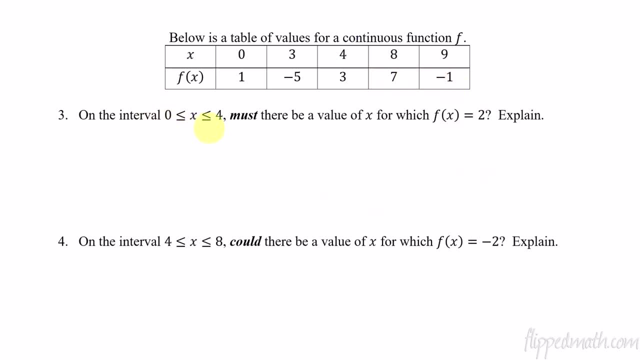 So from there to there, however, you've got to appear somewhere along the way. Next up, we have an interval from 0 to 4.. Must there be a value in which f of x equals 2?? And let's explain. 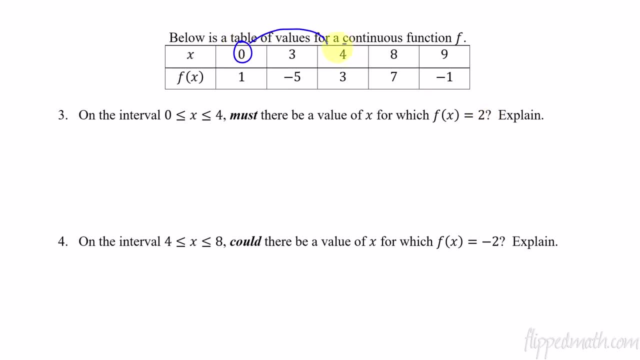 Okay, so we're going from 0 to 4, and does there have to be a point at some point along that way where y equals 2?? Well, we're starting at 1, then we're going down to negative 5, and then all the way up to 3.. So, yeah, there has to be a time somewhere. 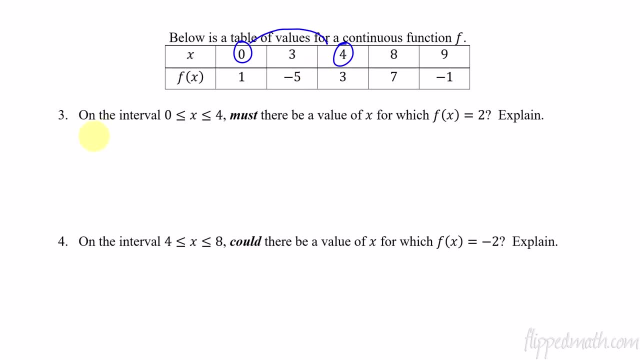 in here where it's got to equal that. so what I'm going to show here is: let's just show that f of zero is equal to one and that f of four is equal to three. now we know it's continuous, because it says right here that it's got to be continuous, and so we've. we've shown that one of the y values is: 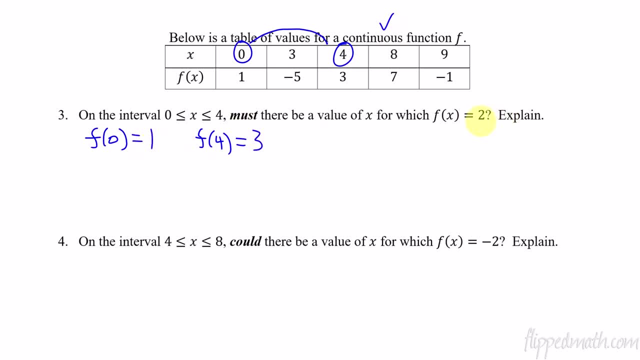 one. another y value is three, and so that number two has to fall in between. so we've shown that it's continuous. we've shown what the endpoints are, and now here's how we do our justification statement. we would say that, according to the intermediate value theorem, there is a value c 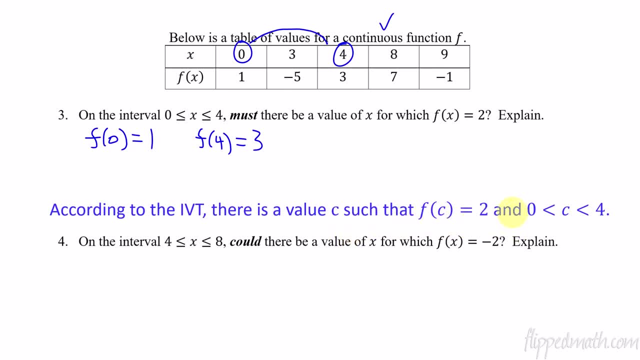 such that f of c equals two and that letter c is somewhere in between zero and four. this is just showing the quick little work. we show what the what the values are, and this is our justification statement, something like that that proves it using the intermediate value theorem. okay, so now how? 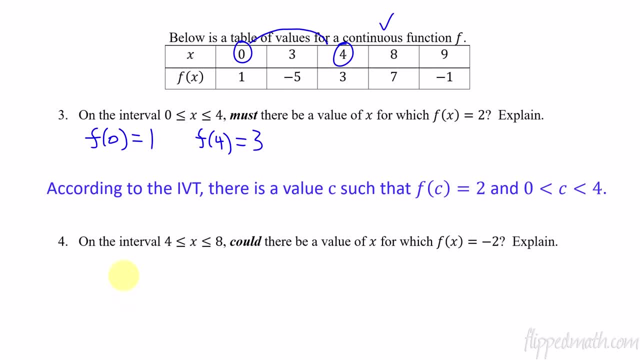 about number four. this is one that I wanted to show you, something that's kind of interesting. you wouldn't see a lot of these on an ap exam at all, but it's still kind of interesting. so we're going to show you what the endpoints are and we're going to show 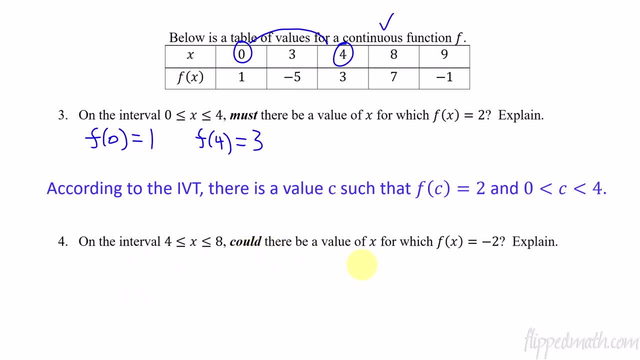 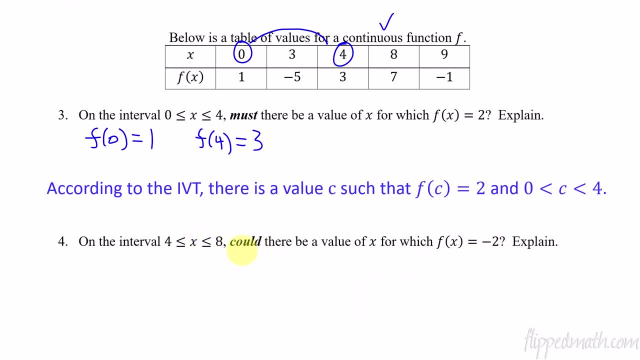 the y value equals negative two and the keyword here is: could not must. so if we look from four to eight, we're just going on this interval right here, from four to eight. on that interval the y values go from three to seven. so from three to seven there's no guarantee that the y value is. 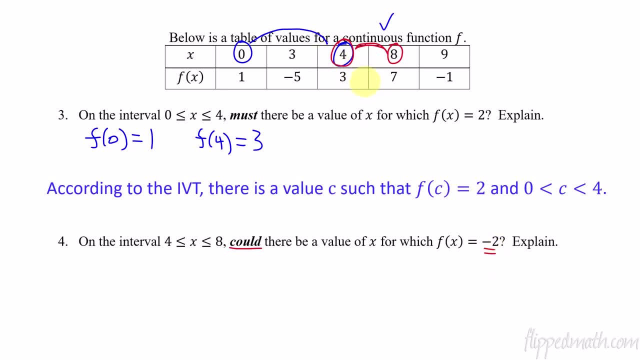 going to hit a negative two. right, we don't, we don't have, we don't know for sure. but what I can do is go up here to seven and every y value. so the y value of three, y value of seven, every y value between three and seven must exist. we don't know for sure what the graph is doing, so I wanted. 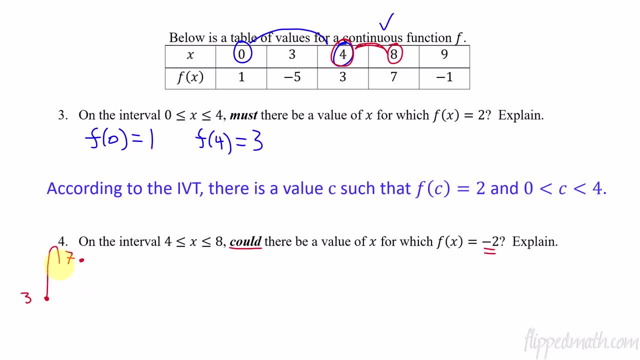 to show you is the graph might be going up like this: past seven, way down here below seven and then back up to seven. we don't know for sure what's happening, so could it be negative two? yes, so this is just a quick little statement that I would put for these, and that is: there's no guarantee that f? 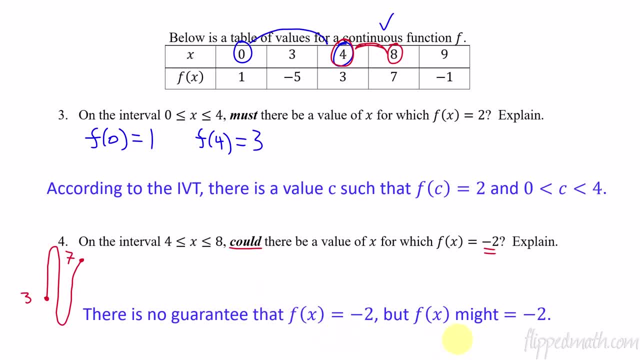 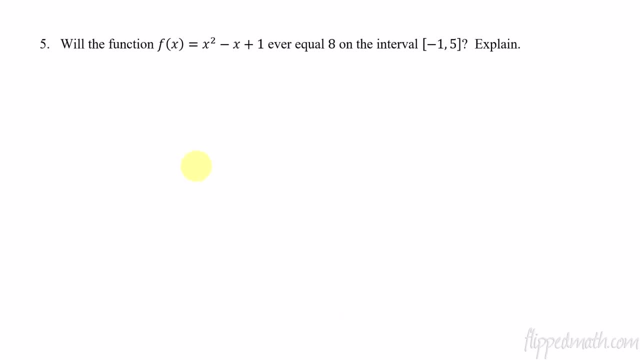 of x equals negative two, but f of x might equal negative two. okay, so the, the intermediate value theorem, cannot guarantee us that there's a negative two on this one, okay. last problem, and this would be a problem more similar to what you might see on, uh, on an ap exam, and that is: will this function ever equal eight on the interval? 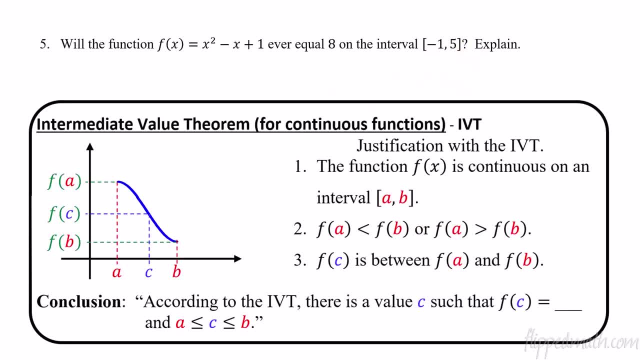 negative, one to five, all right. so let's remind ourselves of something before we do this. there's all of our justifications. that we're trying to do. we're trying to come up with this justification statement. if intermediate value theorem proves so, we need to first figure out: is it continuous? 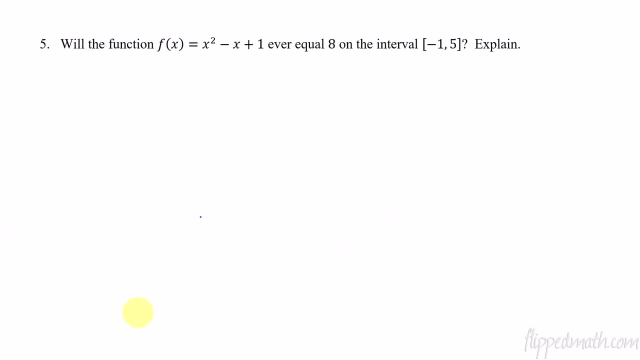 and then we can look at these, uh, the end points there. so is this thing continuous? well, this is a polynomial. so here's what you could say: f of x is a polynomial. and then I can say: therefore, that's these three little dots. that just means therefore. it's a quick way of mathematical talking. therefore. 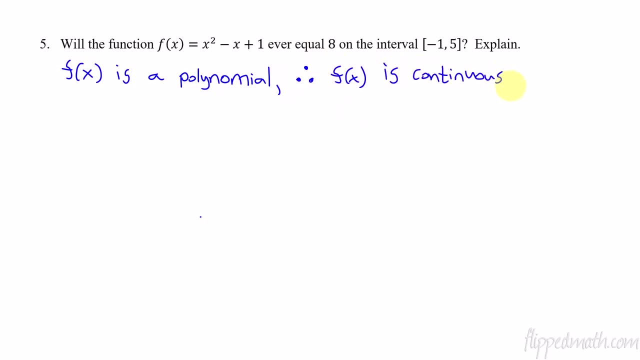 f of x is continuous. now why do I get to do that? we've already shown in years past that polynomials are continuous. we don't need to try and prove that a polynomial is continuous in this case. so we know x is continuous. so there's our, our first condition. we've got that. now let's look and see what are the. 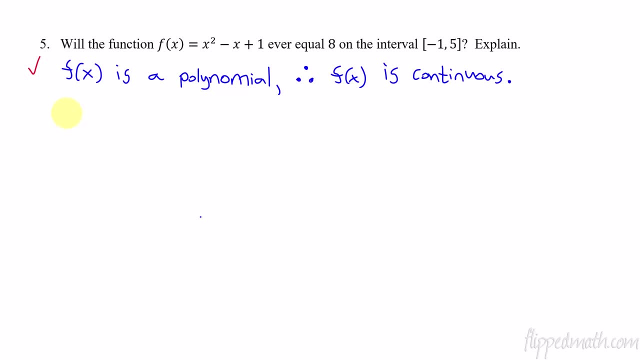 end points here. let's plug in the negative one and the five on the interval. so plug in f of negative one and we get negative one. squared is a positive one minus a negative one plus one. so f of negative one is going oops plus one, f of negative one is going to equal three, okay. so how about f of five? 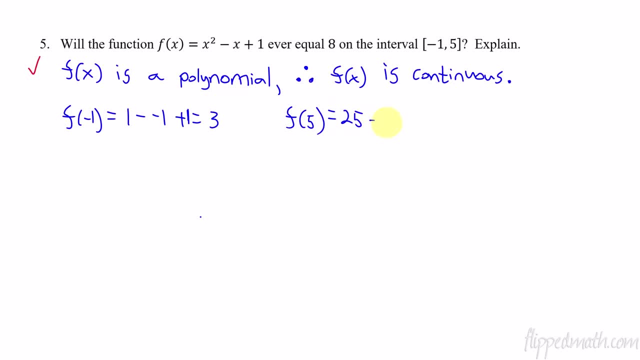 plug in an f of five into these three spots, we get 25 minus five plus one, and that equals 21.. so we're going to be at a value of three, a y value of three on the left side and a y value of 21 on the right side. so is that going to equal eight? yeah,